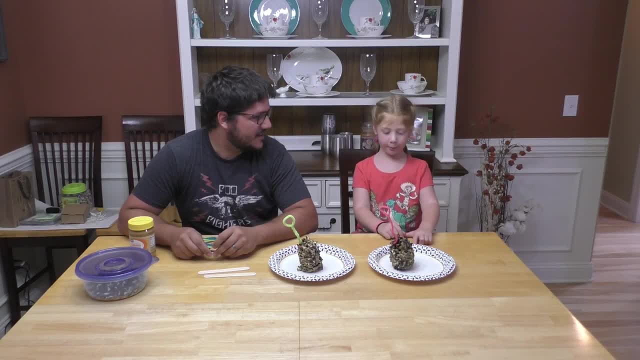 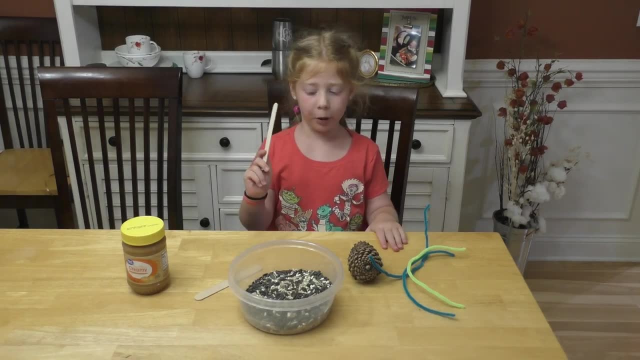 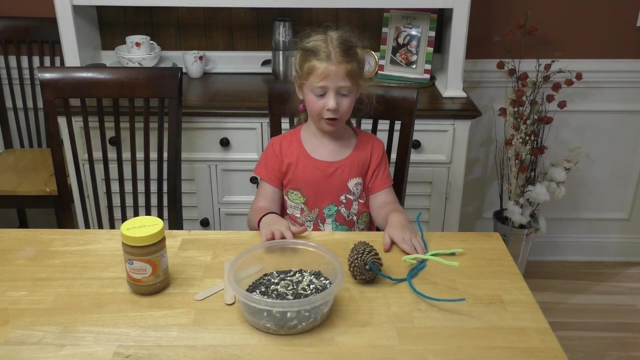 That's right. Today we are going to make pine cone bird feeders. The things you need to make this is popsicle sticks, peanut butter, bird feed, pine cones and pipe cleaners. You might want to wear gloves because the pine cones might prick you. 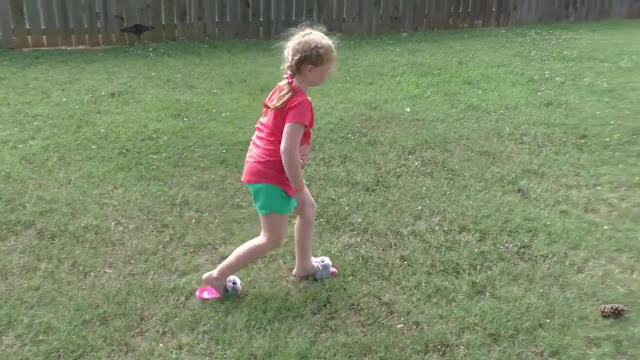 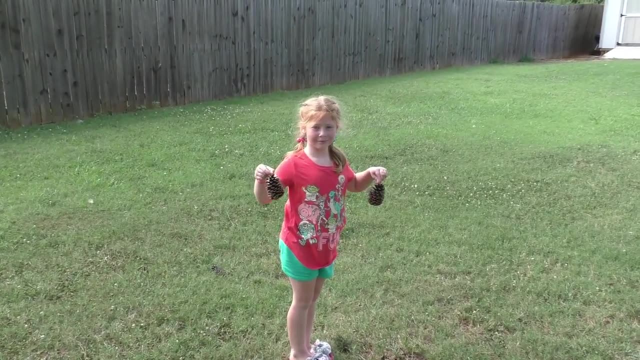 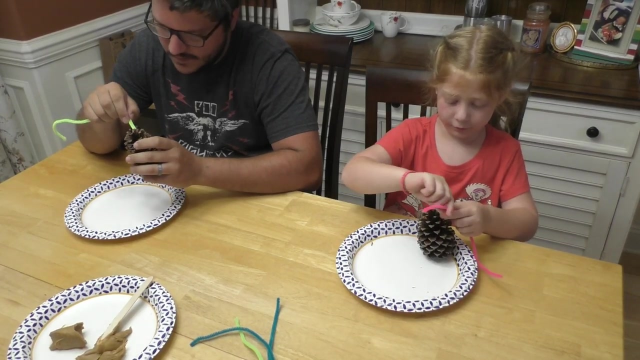 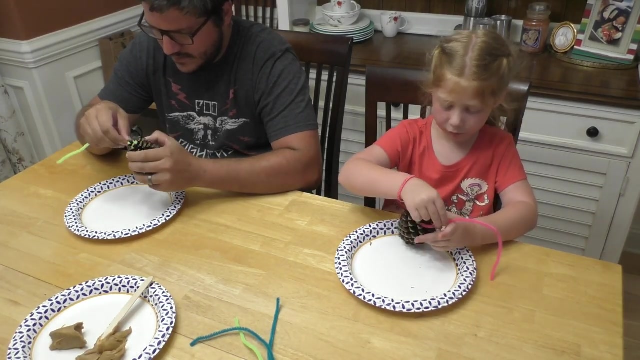 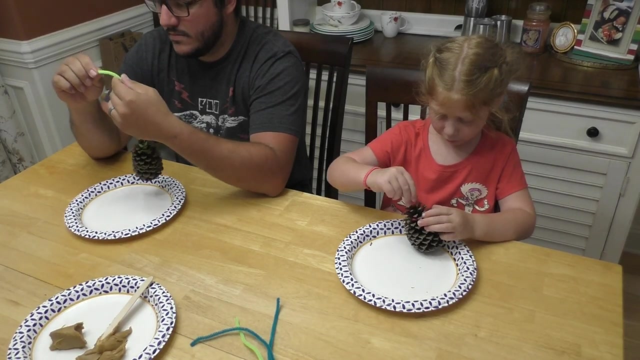 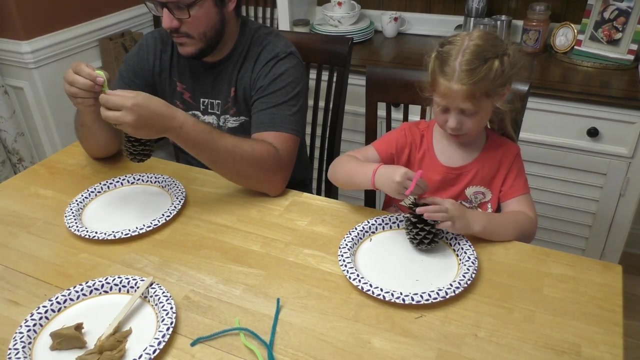 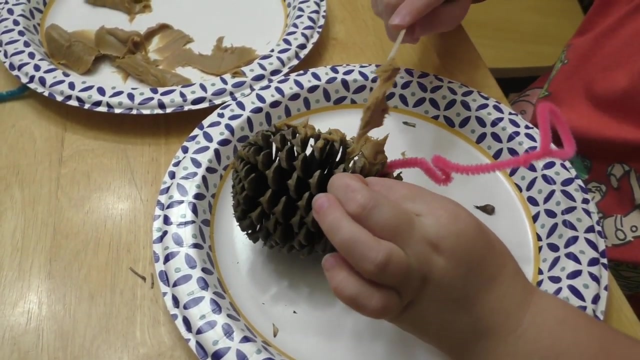 I walked around in my backyard until I found two pine cones. First we tied pipe cleaners on the top of the pine cone. You have to be careful because of the prickles They might hurt. When I was done tying it around the pine cone, I spreaded peanut butter on it. 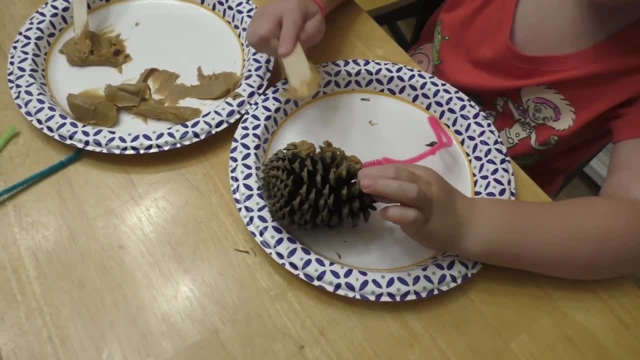 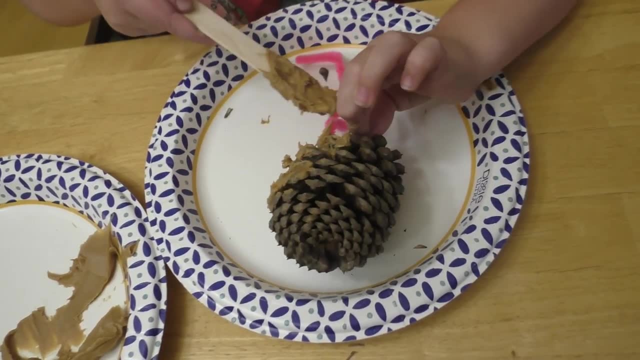 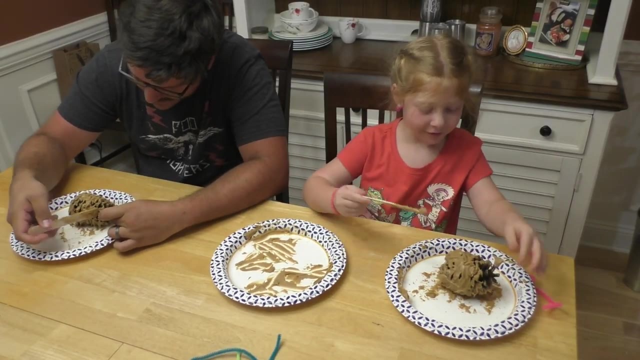 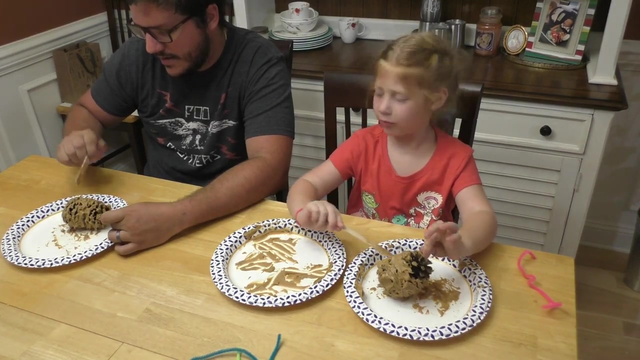 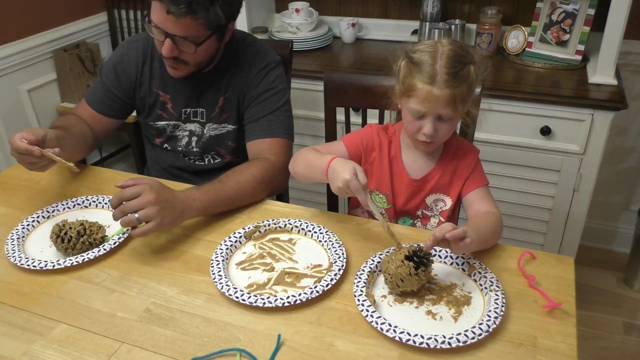 It's okay if you get some on the pipe cleaner, Make sure you get some in the gaps. Just make sure you get them in a group. Then you have to clean them up. We're going to make the pine cone. We're going to make a hole in the pine cone. 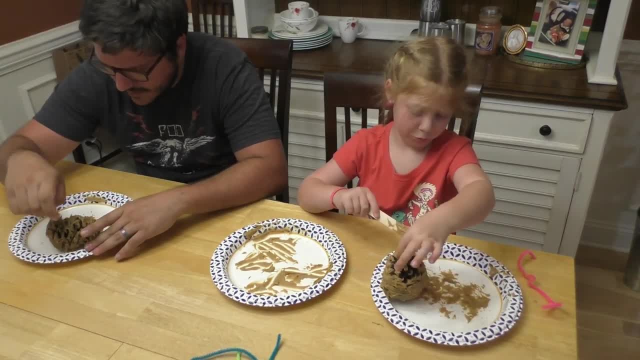 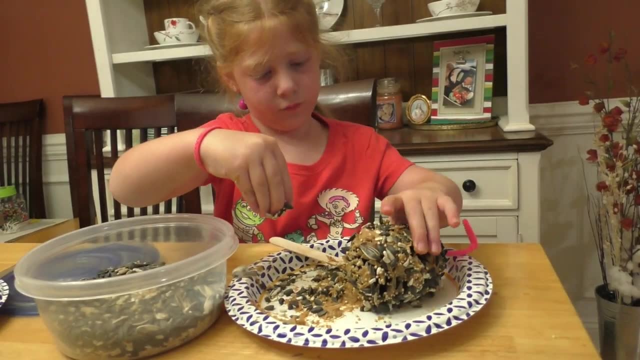 We're going to make the hole into the pine cone. When we are done, we're going to put it on top. I put a straw in the middle of the pine cone To help the pine cone grow. I made a hole in the middle. 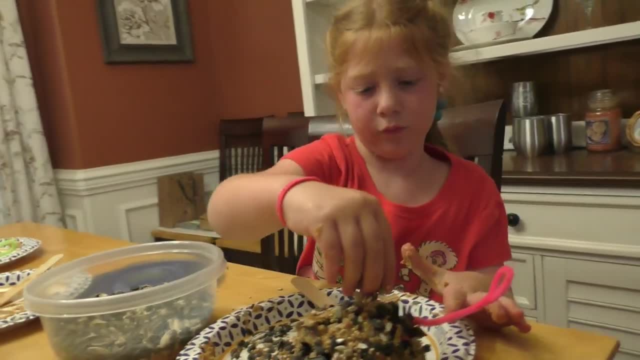 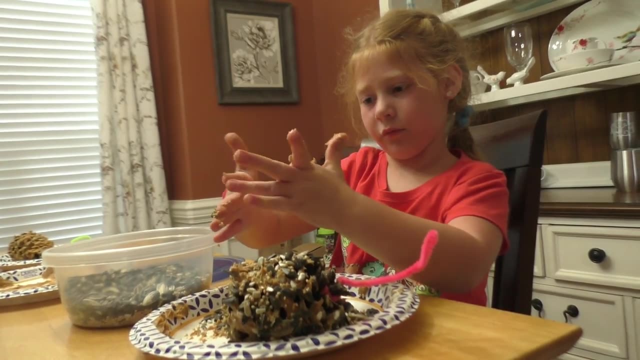 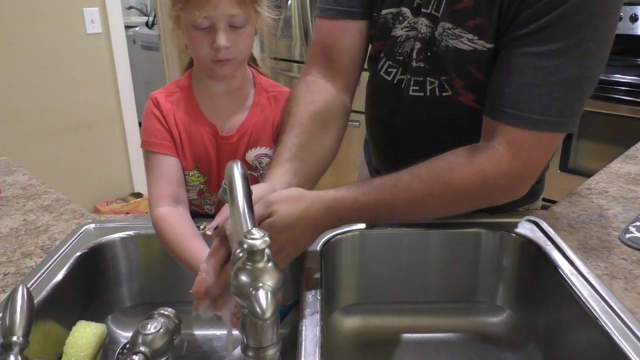 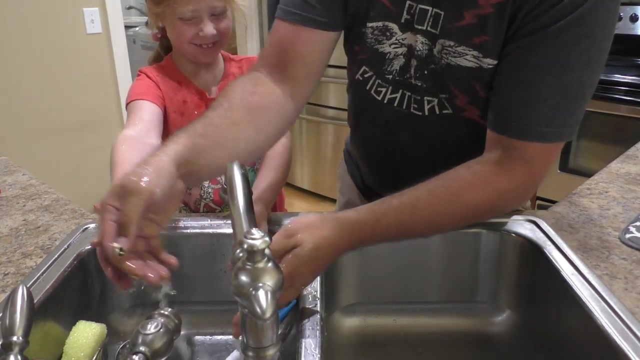 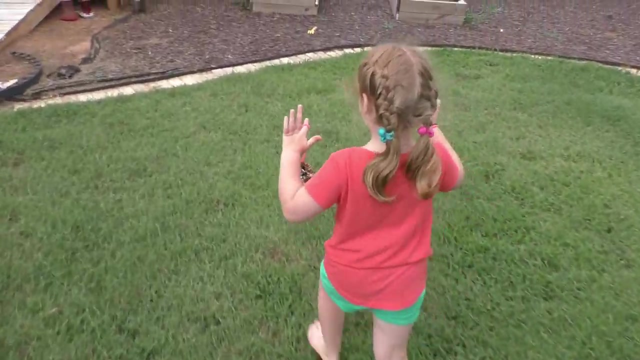 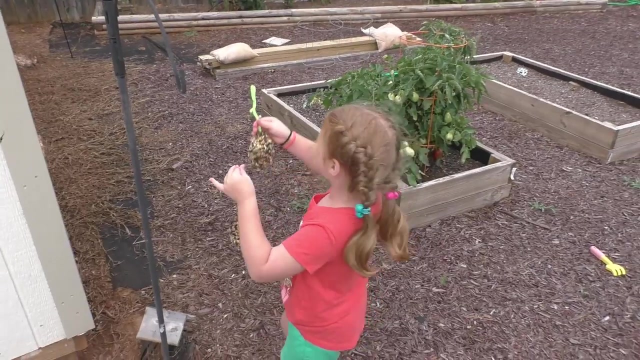 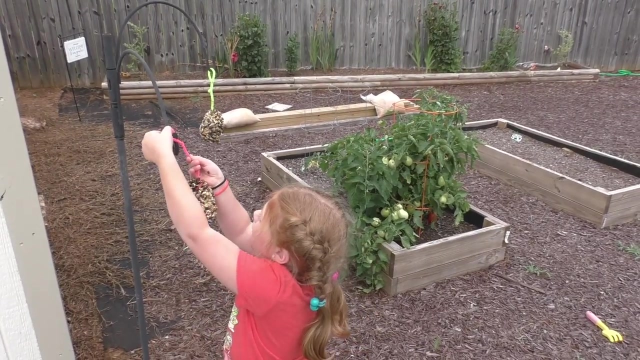 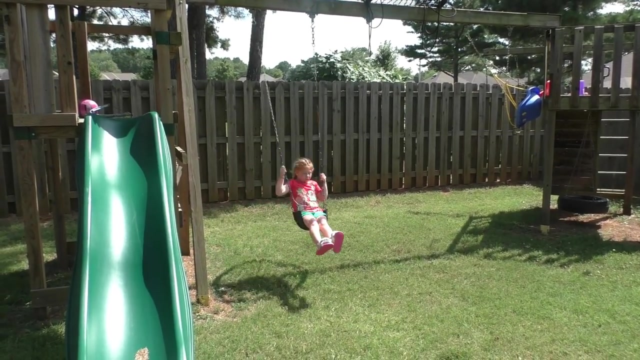 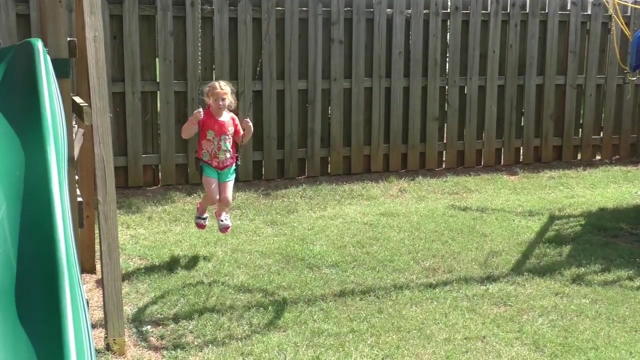 Thanks to the Efens. I didn't set it up and we're all done. when you're done with that, wash your hands. then I hang them up in our backyard. I really like this pinecone bird feeder. thank you for watching with me, you.